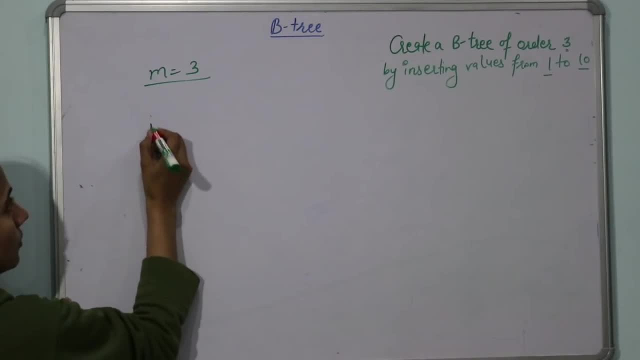 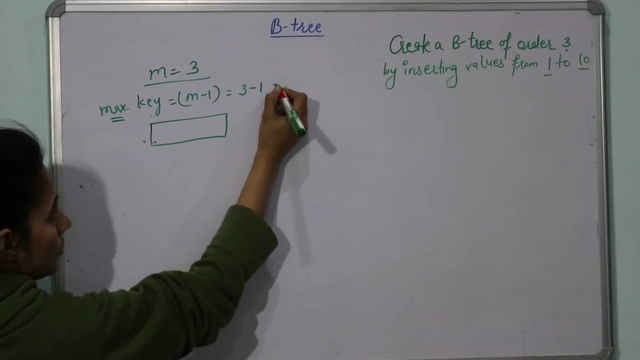 Now start. Let's start inserting. We have this node. How many values can be there in this? How many maximum keys can be there For every node? m minus 1.. You know this from the properties that I discussed in the last video. I hope you have seen that video. That is 3 minus 1, that is 2.. So maximum keys would be 2.. 1 and 2.. 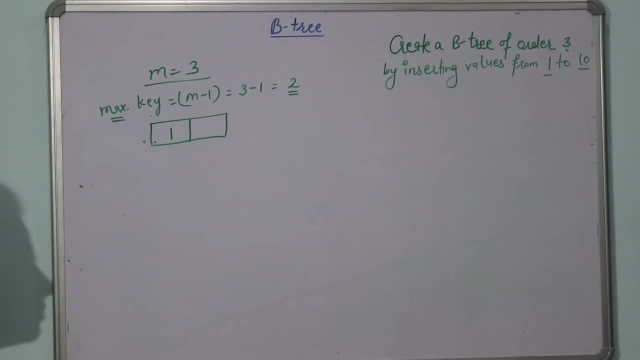 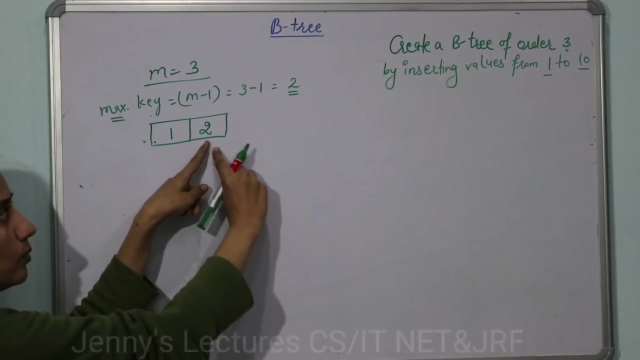 Key 1 and key 2.. Now 1 will be inserted first, After that 2. 2 would be inserted. Okay, And see one more point. These values are always inserted in sorted order. It will not happen that you have inserted 2 before 1. Because this key 1, key 2. So key 1 would be less than key 2. If here key 3 will be there, then key 2 would be less than key 3. And greater than this key 2.. Okay, 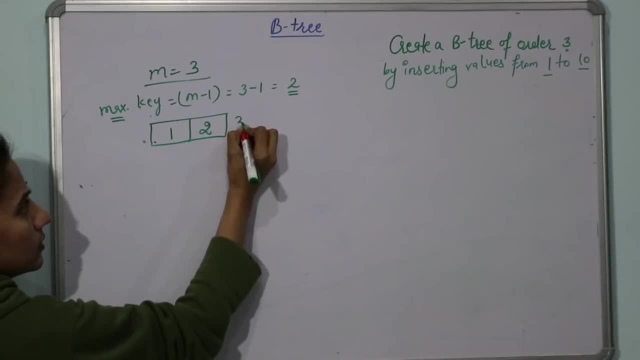 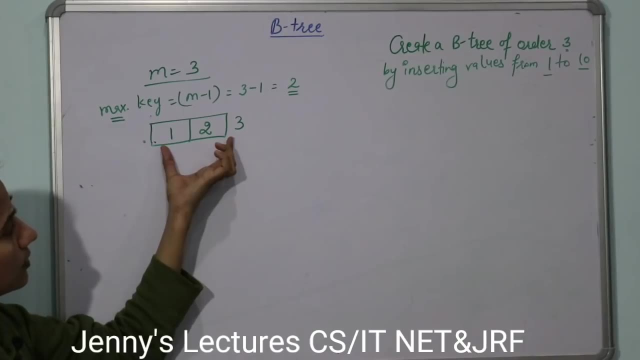 Now see: Next is 3.. You are supposed to insert 3.. But if you insert 3, in that case the value: how many keys are there in this node? 3 keys, But maximum key, how many keys can be there? 2.. So that is overflow condition. Now you have to split it. Now, how will it be split? See: always, when nodes are split, that from where does your median part happen? Or you can say the middle element. 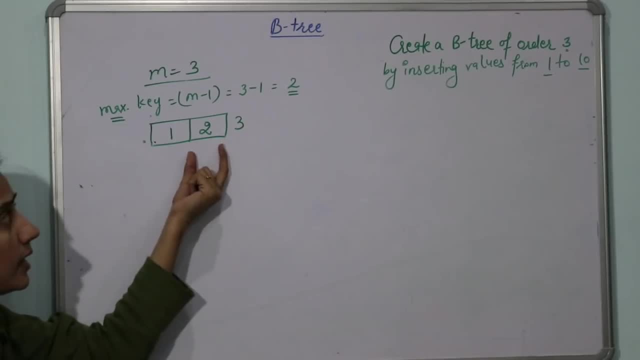 will be calculated first where it is and that middle element would go one level up from this node. one level up, ok, not down. always B tree will grow upwards because leaf node will always be at the same level. now it will not happen that 1, 2 here, 3 insert without you finding out the middle. 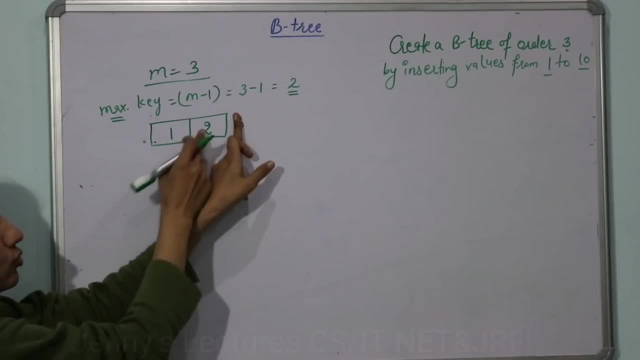 element. find out Kaliya, suppose one year to he can he say be apneus. co. median element: calculate carcass co-oper based, ya know three co-op. consider karoge: uske body of his co-man is committal element. calculate karoge: now the middle or the median element would be two. now this two. 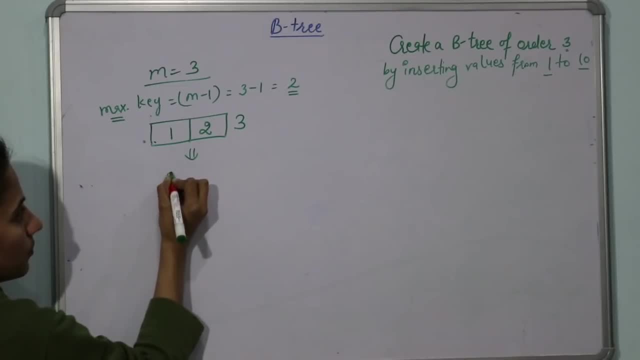 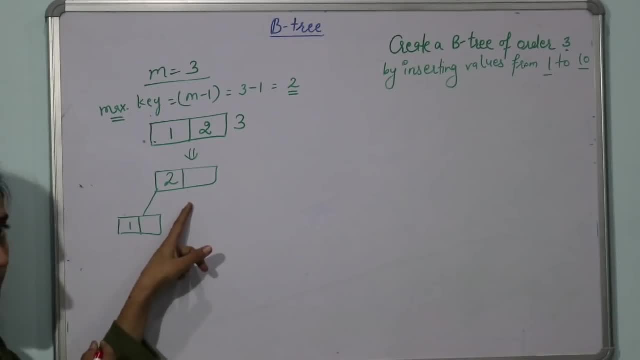 because one is less than one, because one is less than one, because one is less than two. okay, it is see BST, basically generalization of BST to binary search. make a hotel- yeah page, or root hookahs, kill left side. may value would be always either less than or equal to this one and right side. 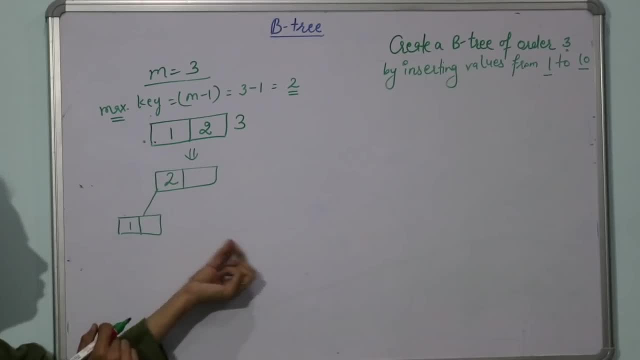 may really would be either equal to or greater than the root node. okay, now to care. right side, make a hookah. three, though. hey, a box is because maximum key kidney insert. also. okay to now the next key up. good insert, Kanye, that is three-tech insert. oh yeah, next is for root. 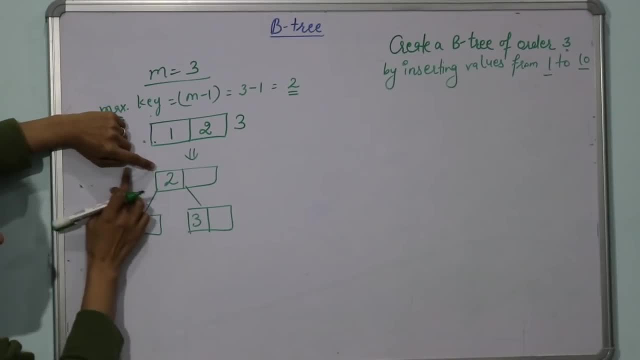 peg ECE, insert a mashaka, serve a leaf nodes, but they can get them pass a root node, say four is Oh, greater than two, so you have page hanging. but up here hop a insert nahi caroge. although the this place is, you know, empathy, you can insert, but from insert is many cups up there, because 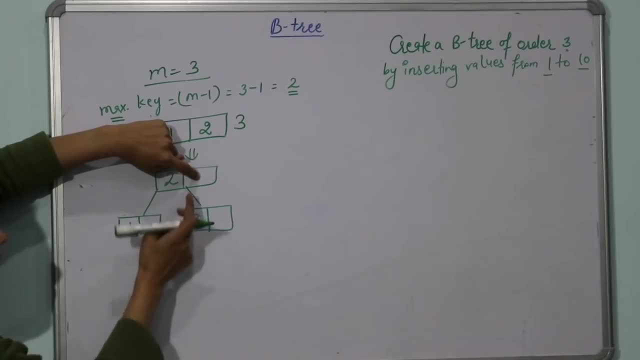 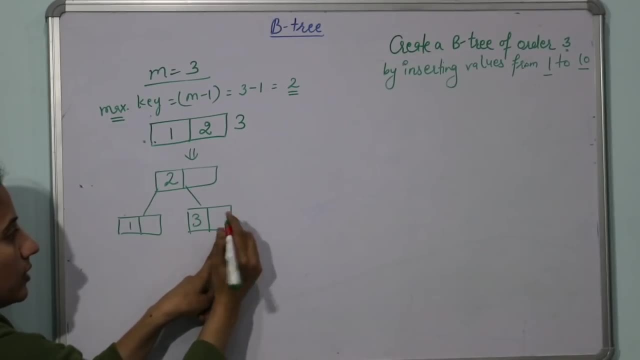 well you can't be inserted, or Tameesha leaf node way. so is care right part many change jayenge. that is three, three say be, but I have four, so yaha pe insert ho jayega, because it is leaf node, is k niche kuch bhi nahi hai to yaha pe apka four insert ho gaya hai. next value is five a five. 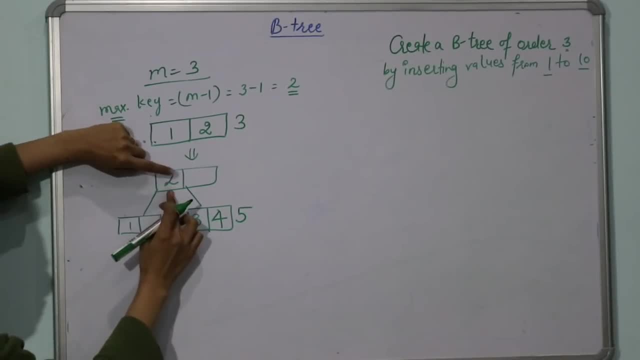 agar insert karni hui to wo yaha pe insert hogi. because two say always five is greater than to hum yaha pe gaye. three say greater than greater than four, to five apke kaha pe aayegi, yaha pe aayegi. 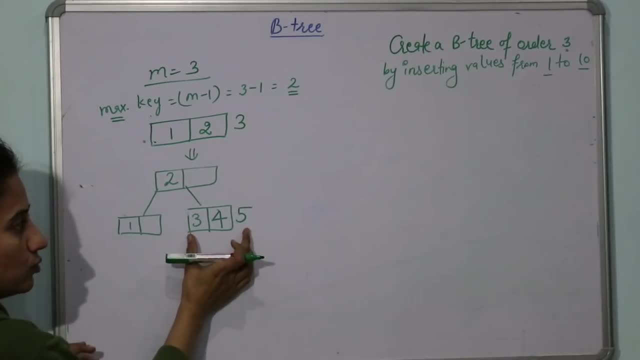 but maximum keys can be two and here we have three keys. so this node would be: you know, we have to split it. split kyaise hoba. first of all, middle jo, median element. hoe find hubab, find out hogar. and that median element or middle element would go to one level upper. you can say the to the pair. 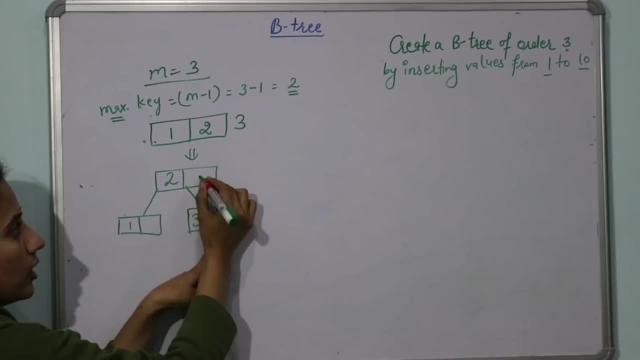 parent of this node. parent is kahaye roto four. kaha pe chalage apka year hape jayega and see tree kya bun jayega apka two, Then 4. Here we have 1, See and 3. 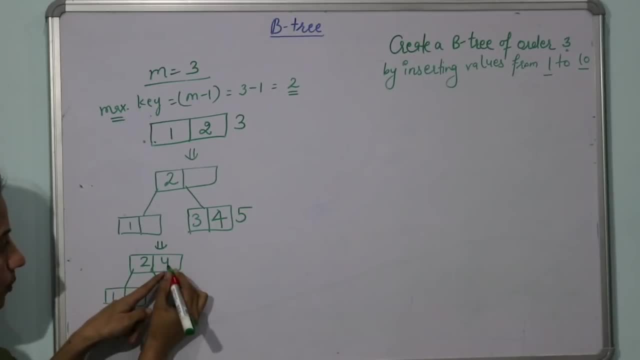 Where will it come After 2? but to the left of 4. Here it comes 3 and 5. Where will it go right of 4? Because 5 is greater than 4. So it will go to the right And 3 will be to the left of 4. 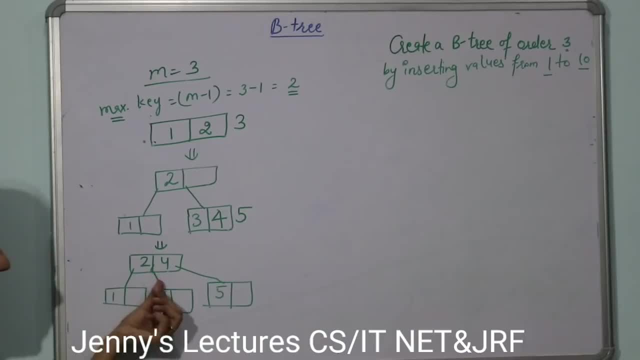 Because it is less than 4, But it is greater than 2, So it will come to the right of 2 and left of 4. Now, next we have to insert 6 Here. 6 is greater than 2 and 4, So it will go to the right of it. 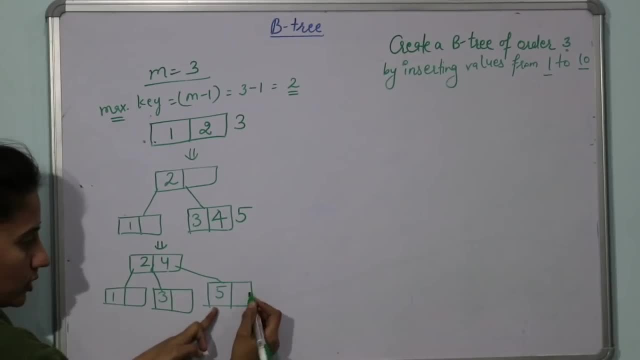 Here we have leaf node. One position is there That is vacant, So here 6 will be inserted. After that 7. 7 should be inserted here, But we cannot insert it here Because, Because we have to insert it here, Because we cannot insert it here. How much maximum is it? 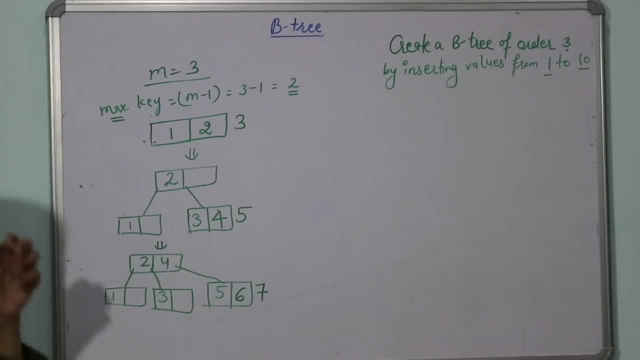 It can be 2. Now again, this node would be Split. it Split from where Median element, That is 6, Where 6 will go 1 level up, That is to the parent, Now 6 If it goes here. Ok, So that is also not possible Because here is already full. 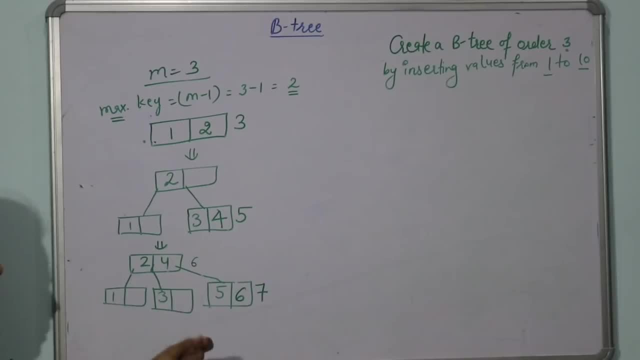 It can be of 2 And what happened here, 6. So again, Splitting will be applied to This parent of this one, or you can say the root 1. here the split will apply. we will find out the median element. what is the median element of this 4 and 4 would go to its parent parent. it has nothing. 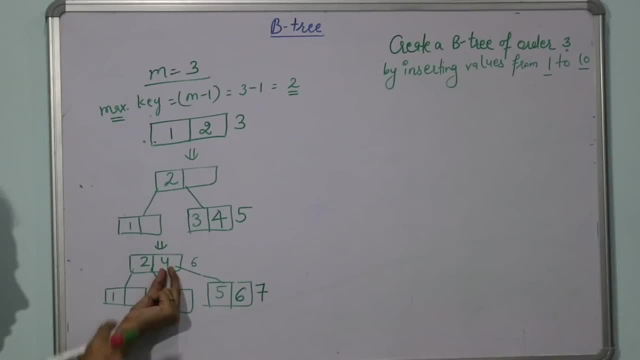 so this is your one level up means this will be your second root. ok, now what will be next going to be? What will you make the tree of ours? the tree would be: 4 has been split from here 4. what will happen on the left side of 4? 2? 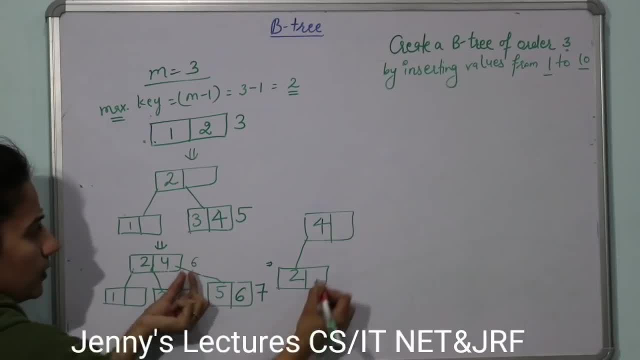 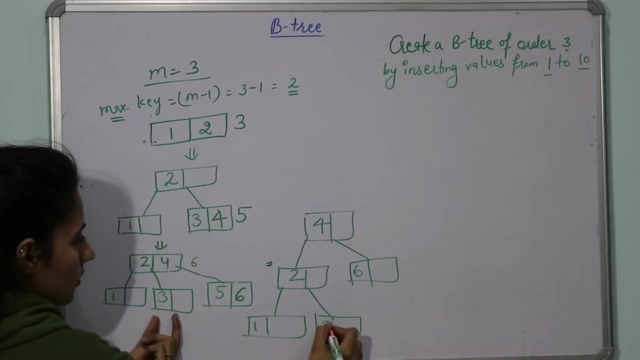 what will happen on the right side of 4?? What will you be here? six, ok. now see what do you have on the left of 2? 1. ok, ok, impact on 15. 12. 12. 2 ke right mein, what you have is 3, okay, and apki 5, 6, apka upar chala gaya 6 yahan to 5 kahan. 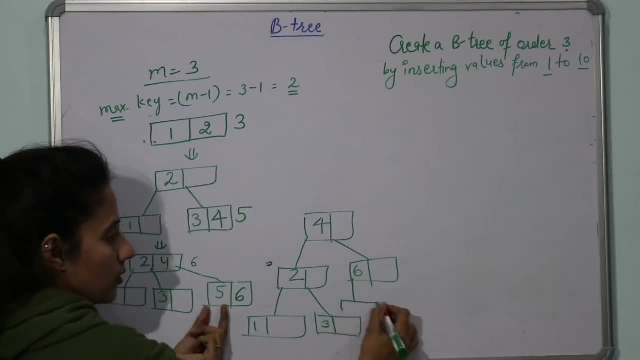 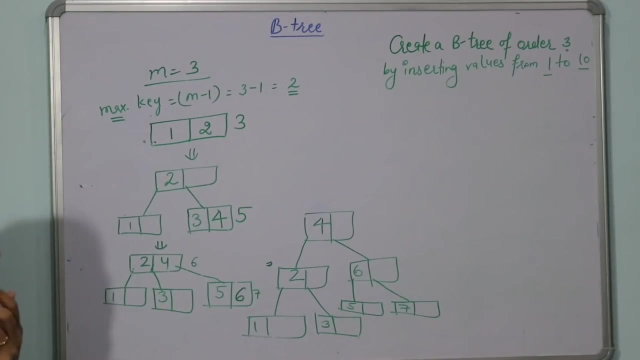 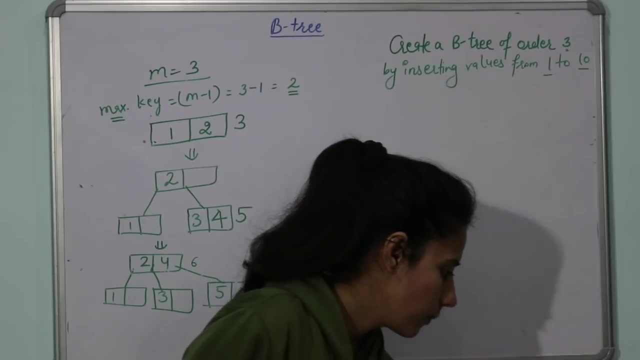 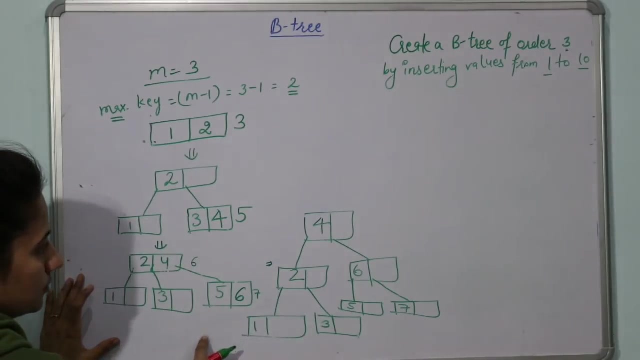 pe aayega apka left of 6, because it is less than 6. 7 insert karna tha 7 apka kahan jayega yahan pe right of this one. okay, now see. now we have to insert what 8, 8 apka kahan insert hoga root. se. 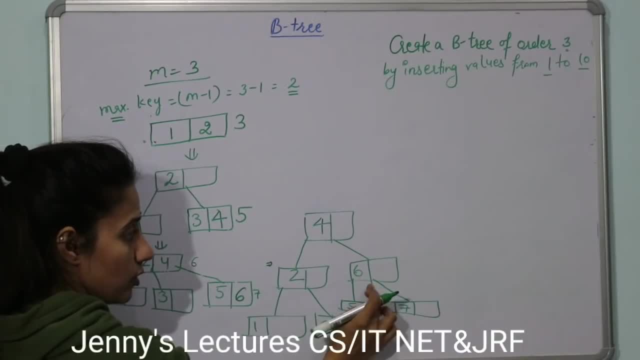 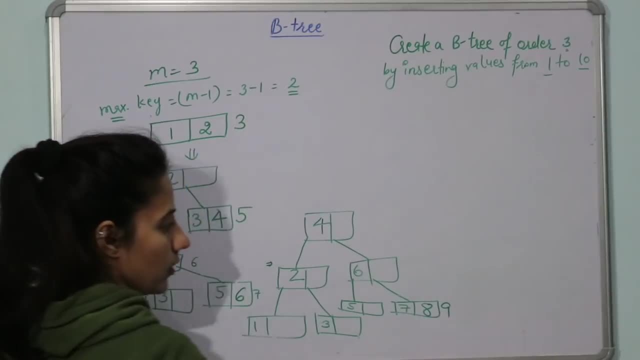 4 se greater than hai. yahan pe gaya 6 se greater than hai, but it is not leaf node wo yahan pe jayega 8 apka kahan insert hoga, hair only now. next is 9, 9, 4 se. 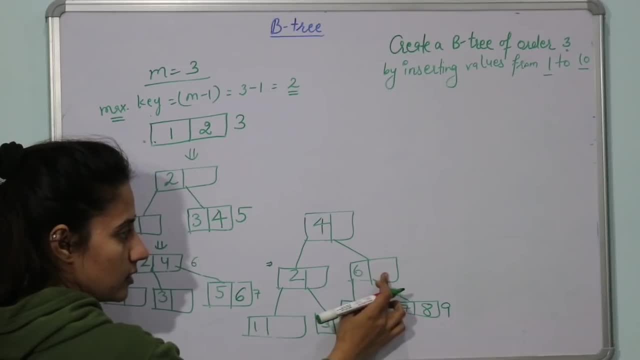 greater than hai, greater than 9, 6 hai. lekin yahan insert hum nahi kar sakte, because always it would be inserted in the leaf node to yahan pe apka 8, ke baad 9, but over flow condition apke paas. 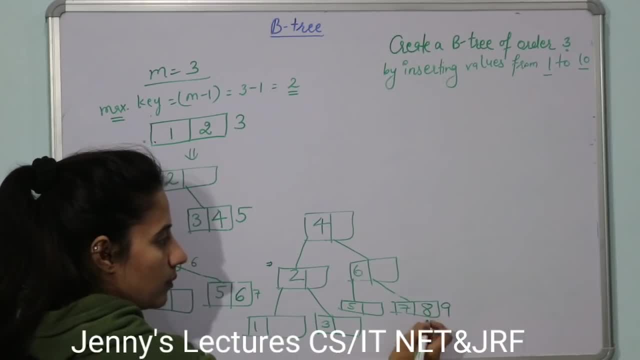 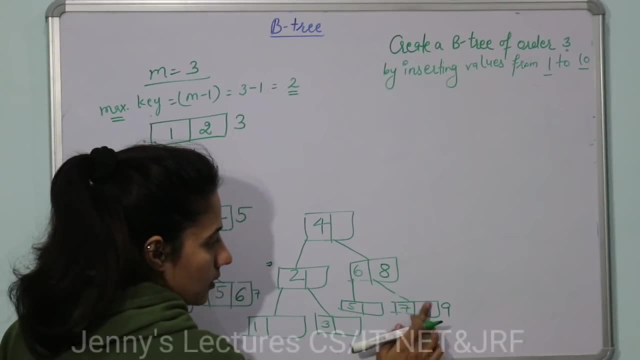 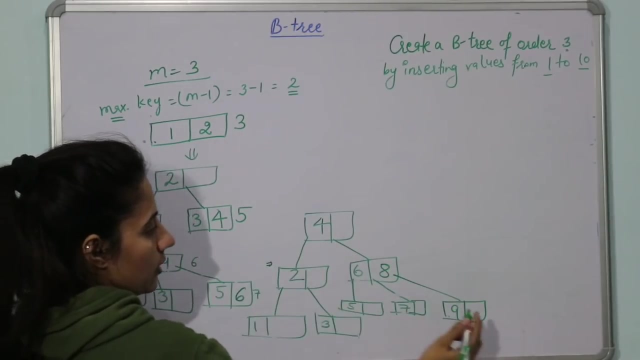 aage yahan pe to splitting. kya hogi 8, apka kahan jayega abhi upar 8, apka chala gaya yahan pe okay, and 8 ka left part would be 7 and 8 ke right me. kya hoga apka 9? okay, and next element is 10 to. 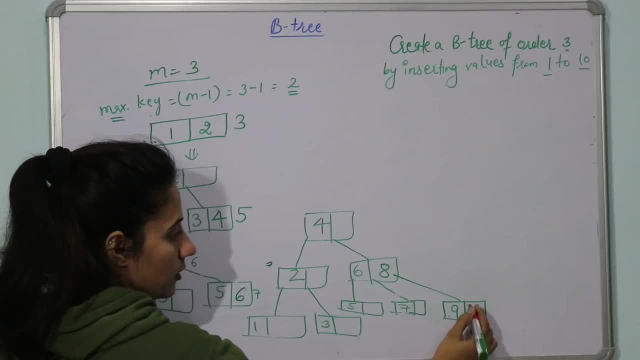 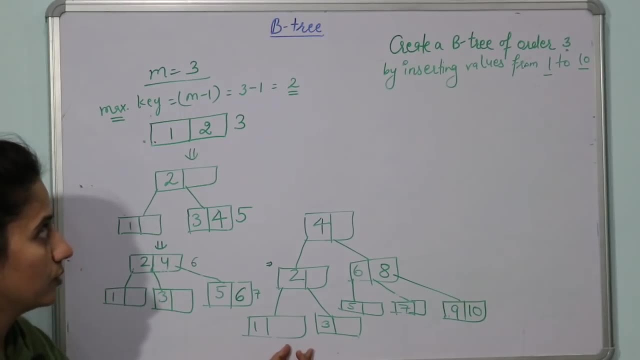 10. apka kahan pe see always humesha aaye kahan pe hoga apka leaf node me insert hoga to 10 would be inserted here. so this is the B tree of you know order 3 and the values jo humne insert ki hain that.